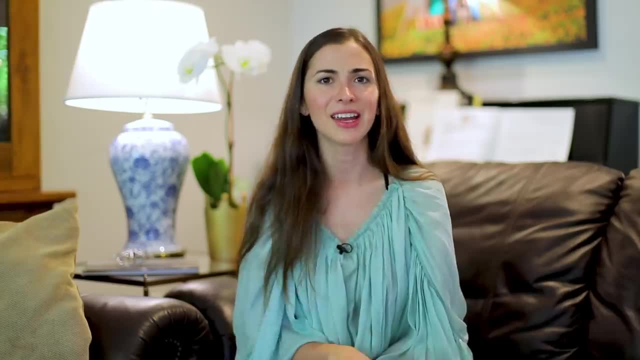 what are your cravings? What are you craving for when you're pregnant? I didn't have any cravings, by the way, but it's just a great phrase to say: I am craving something. You don't have to say I'm craving something. You don't have to say I'm craving something You don't. 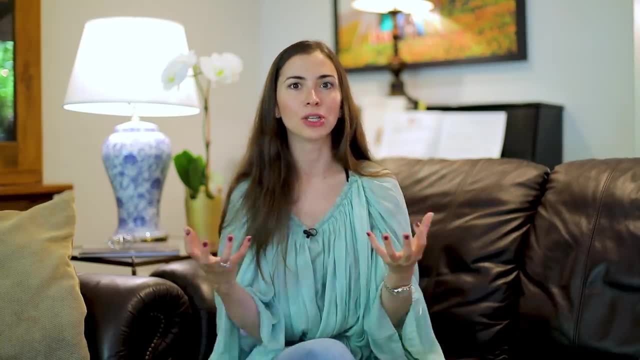 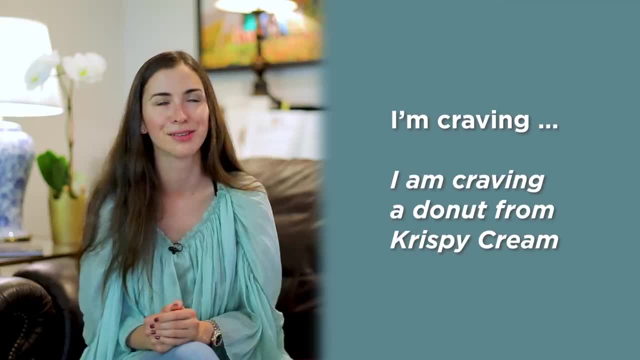 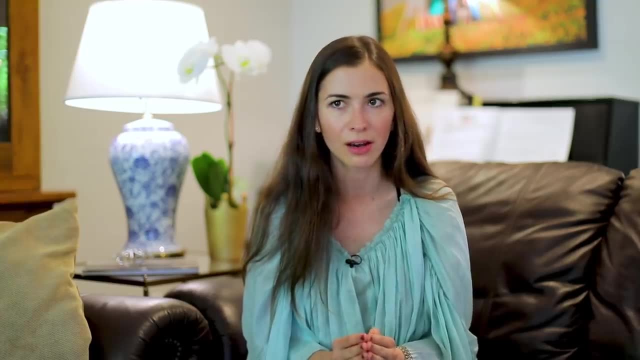 And, by the way, if you try it, it's really unhealthy but it's also good. I am craving a donut from Krispy Kreme. I am craving McDonald's. Oh my God, again something that is really unhealthy, but they just add something to their food that you wanted all the time. Comment down. 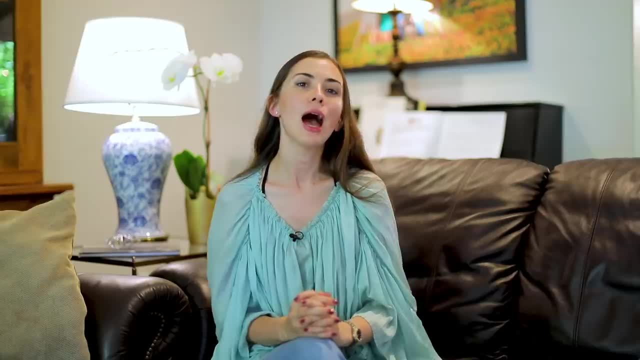 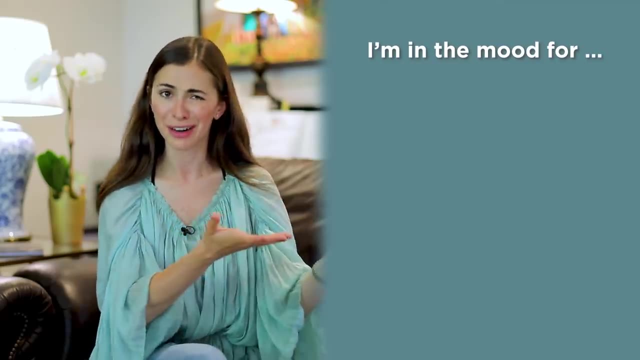 below if that's the same for you. I'm craving some teriyaki beef. I'm in the mood for Again. this phrase is very light and it's used in a situation where you're talking about food again or something that you're willing to do. tonight, For example, I'm in the mood for sushi. Let's go. 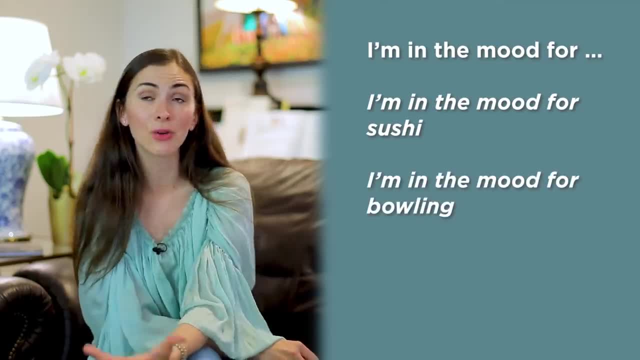 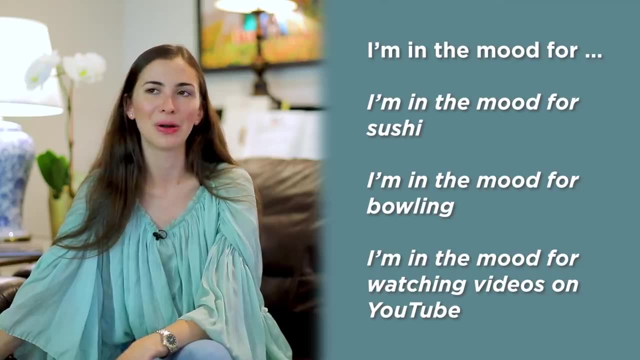 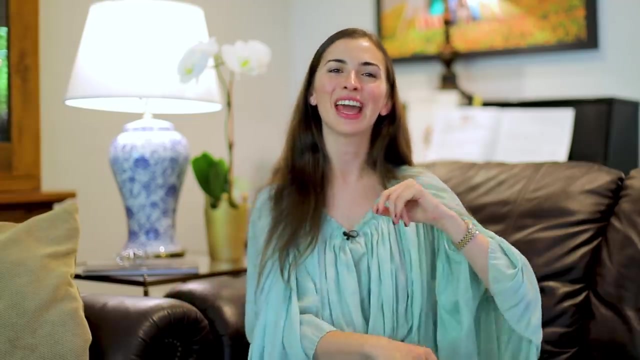 to that sushi place. Or I'm in the mood for bowling. Let's go bowling, which isn't really a reality to many people right now. but I'm in a mood for watching videos on YouTube and staying at home. I don't want to go out tonight. Do you agree that saying I want to watch YouTube is a? 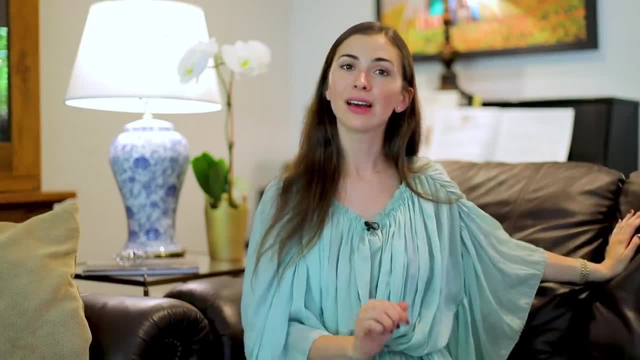 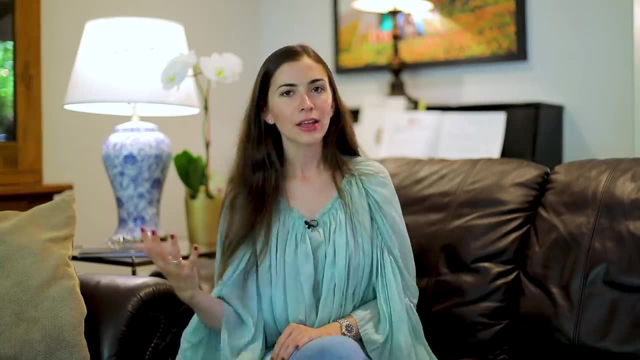 good thing. I'm in the mood for watching a couple of YouTube videos. It sounds a little aristocratic. I like it. I like this phrase. I'm in the mood for some music. 80s- Another phrase that you've probably learned but aren't using that often. I feel like. I feel like eating. 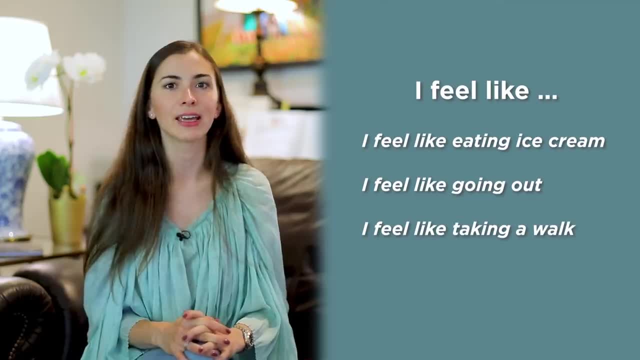 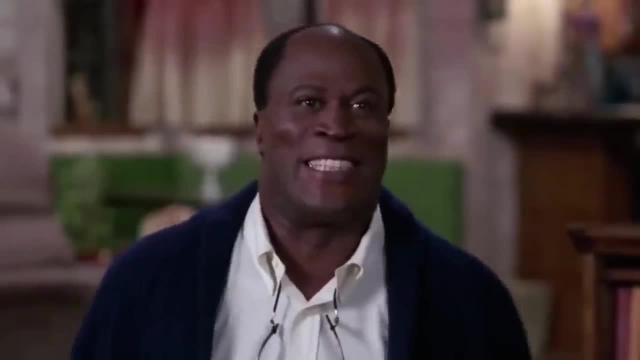 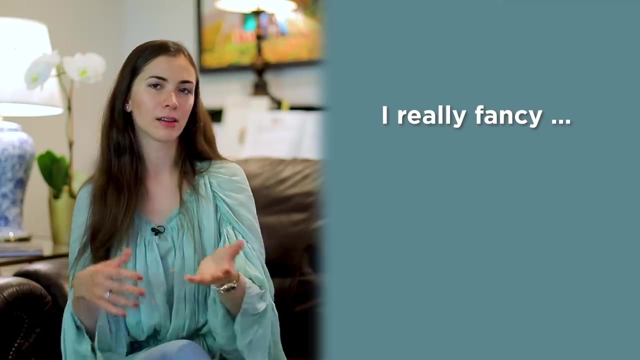 ice cream. I feel like going out. I feel like taking a walk. I feel like watching TV. This is a great phrase to express your desires. I feel like break dancing. A phrase I really fancy has the same meaning as a phrase. I feel like. It means I want, but it's like. 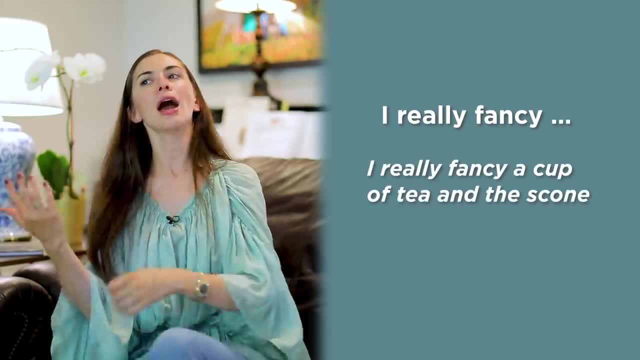 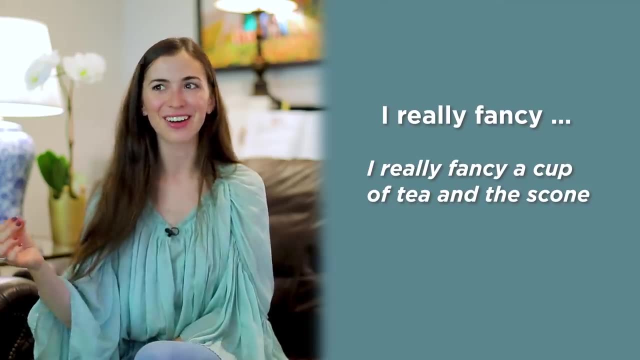 it would be great to have something, And it's mostly used in the UK. I really fancy a cup of tea and a scone right now. This is very British, by the way- Five o'clock tea scone, So I really 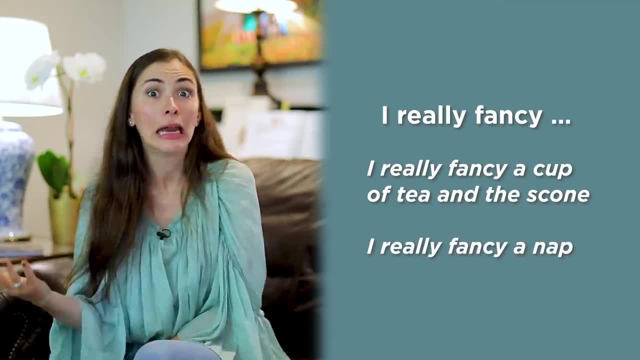 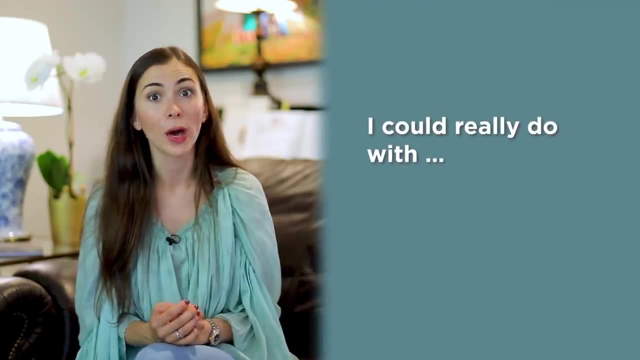 fancy a cup of tea. I really fancy a nap right now. Yeah, I don't really fancy this color. Another way to say I want is to say I could really do with something. I could really do with a cup of coffee right now. By the way, 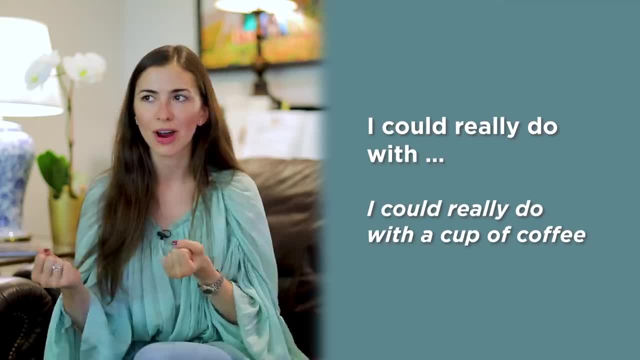 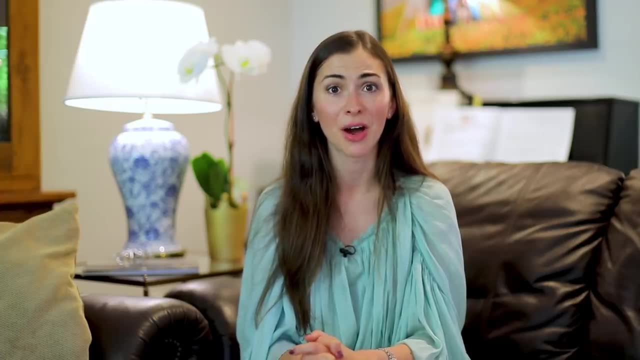 in the place we're in they don't have a coffee maker, So I have to drive to get my coffee, and I just love coffee in the mornings. I really want another one right now, So I could really do with another cup of coffee When you really really want something and you're talking to. 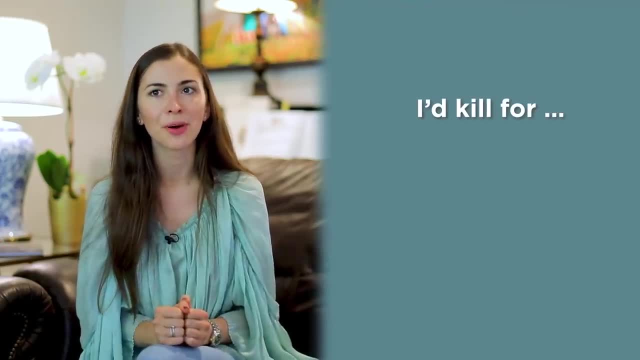 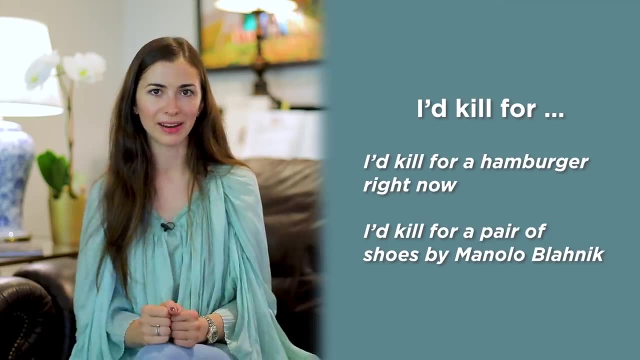 your friends kind of informal environment you can say I'd kill for. I'd kill for a hamburger right now, I'd kill for a pair of shoes, Manolo Blahnik, So something that you really, really want. but remember it's for an informal. 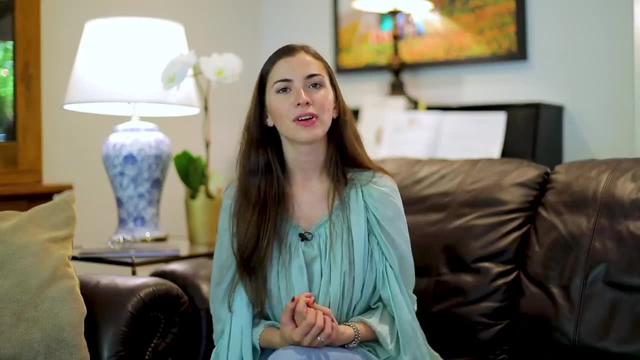 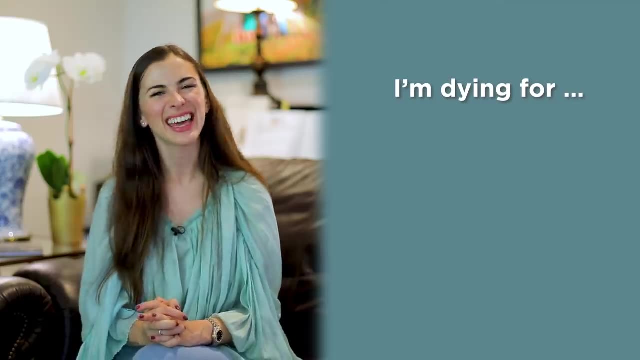 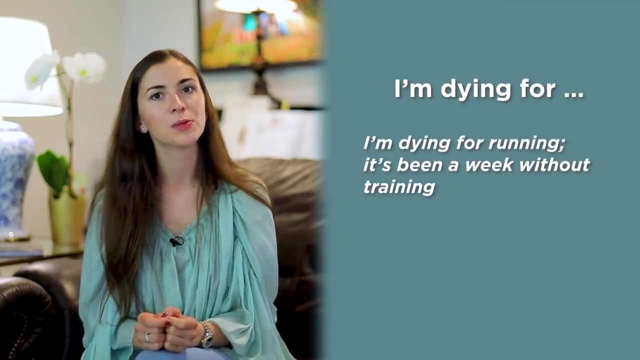 conversation: Oh, I'd kill for a latte. Another phrase is kind of similar to I'd kill for something to do with death. I am dying for- And again this is really informal and this is when you really really like or want something. I am dying for running. It's been a week without. 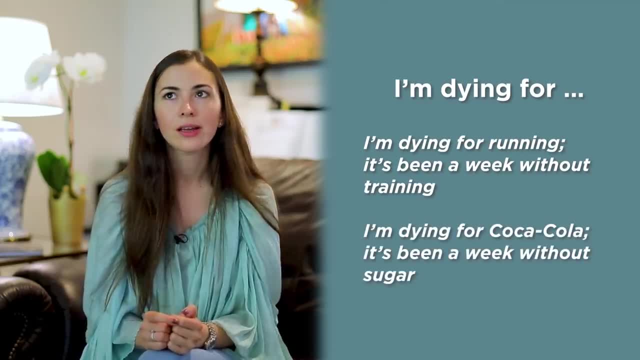 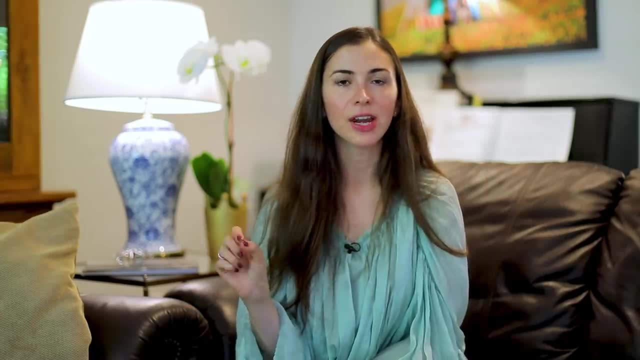 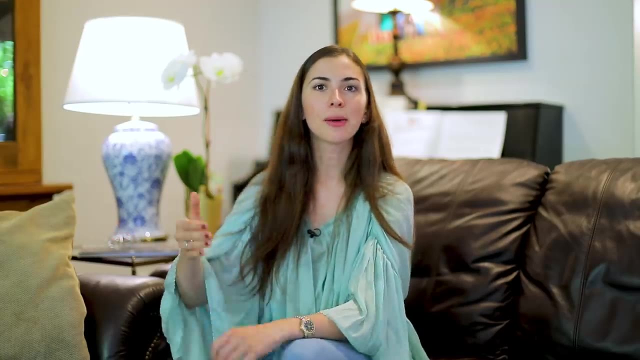 training. I am dying for Coca-Cola. It's been a week without sugar. Yeah, I'm just dying for a drink. The next phrase is really, really useful And it's the last phrase for this video. We use this phrase when we are open to something but we're not committing to it. So, for example, 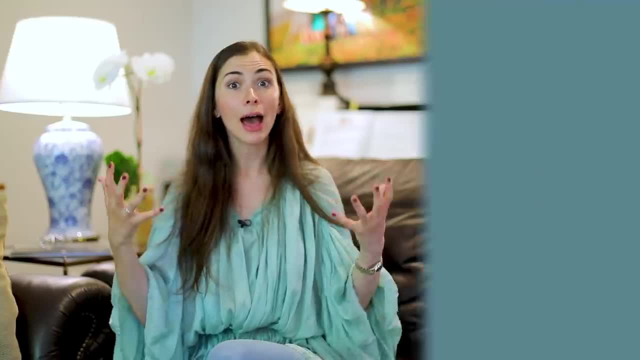 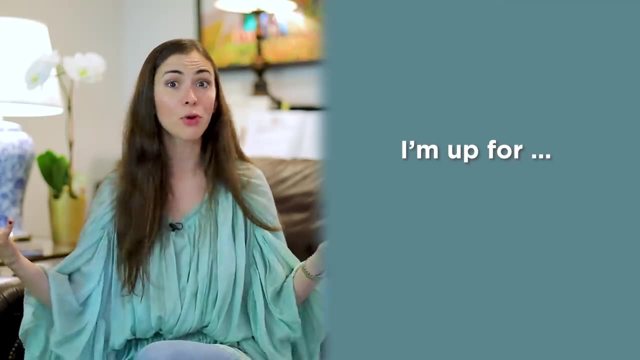 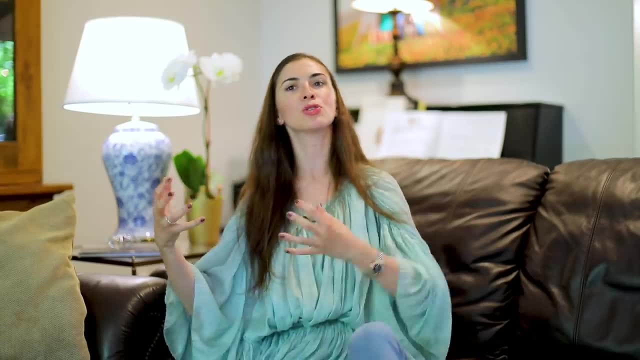 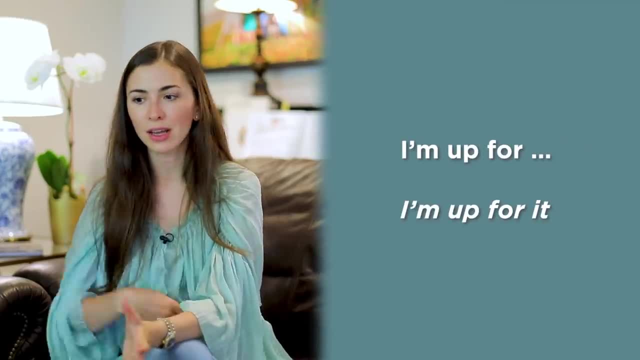 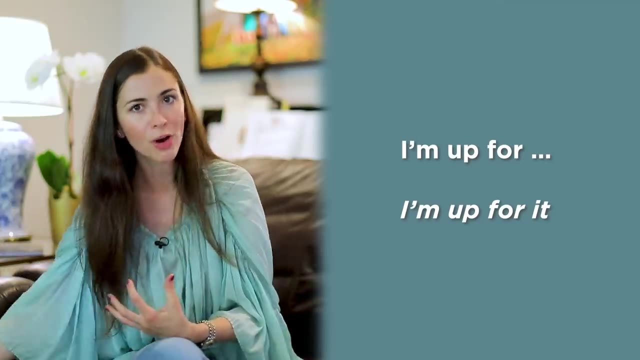 with them and you're like: I'm up for it. It doesn't mean that you're going to start planning everything right away. It means that whenever the other person decides that they want to proceed with this project, then you would jump in. But right now you're up for it, You're not against. 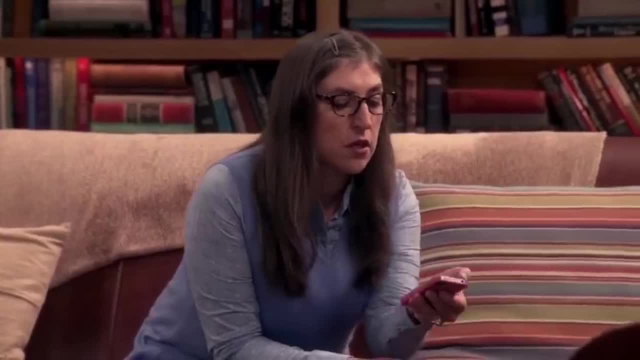 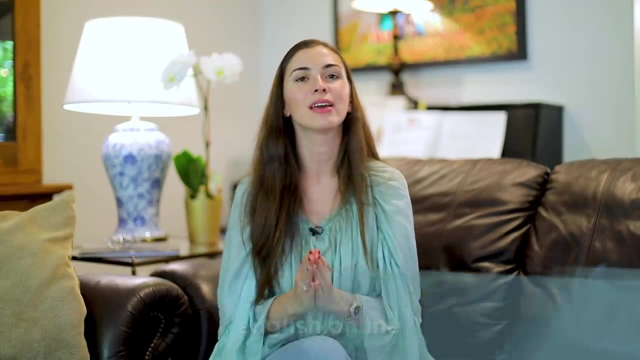 the idea, but you're not jumping on it right away. I'm up for anything. Thank you, guys, so much watching this video up to the very end, As always. if you want to practice more English, Englishonline is a resource where you can buy my handbook for English language learners. It has.